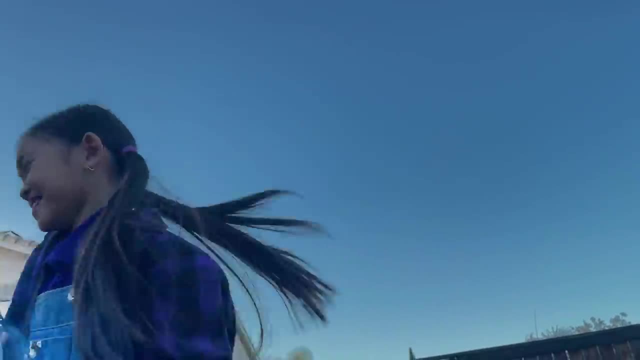 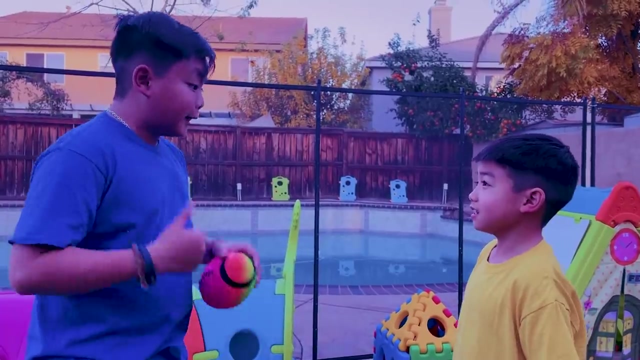 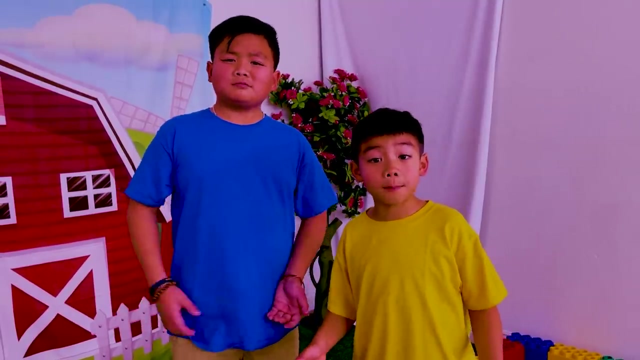 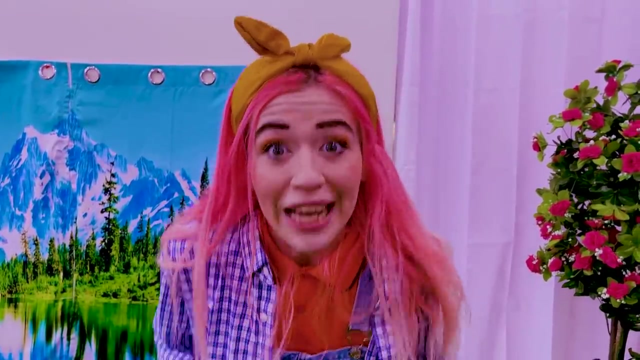 We need a plan to get the sun back. Let's follow her. What happened? The sun is gone. Oh, if the sun's gone, the planes can't roll. That's called photosynthesis. Can you get the sun back from the giant for me, please? I'll let you borrow my plane On it. 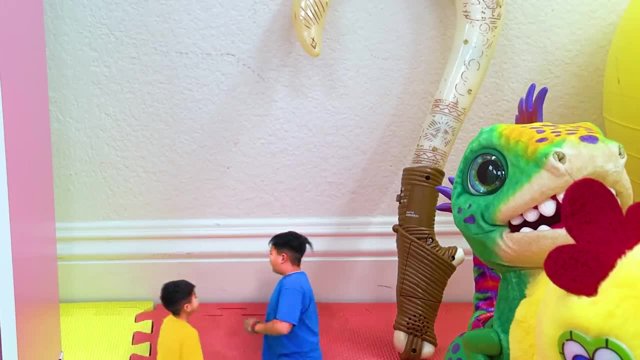 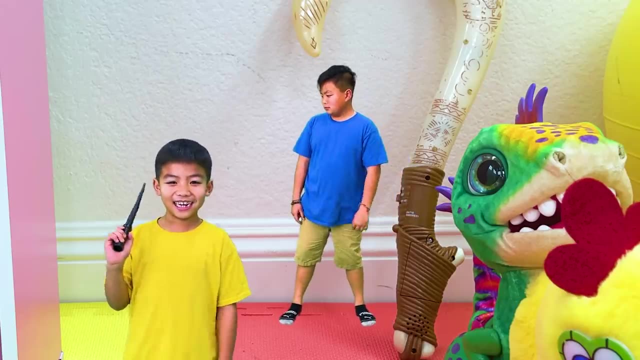 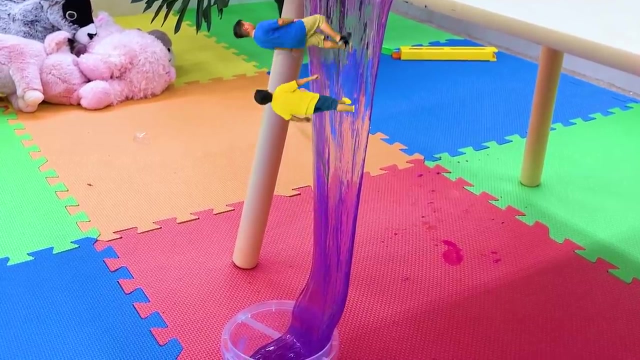 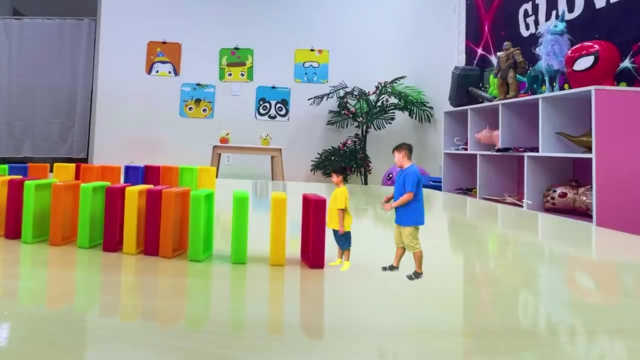 Okay, we're here now, but how are we going to get the sun back? Oh, over there. Wow, I got an idea. Hee-haw, Remember Eric. we cannot let the giant hear us. Cool domino What. 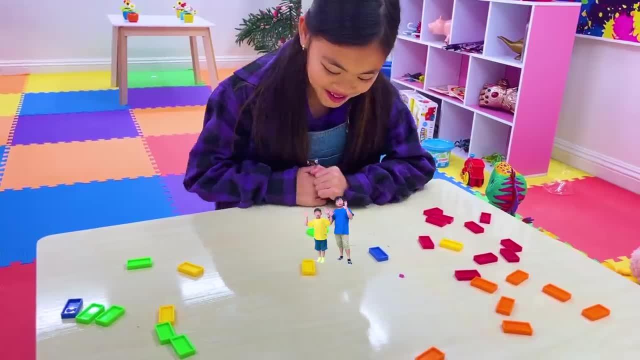 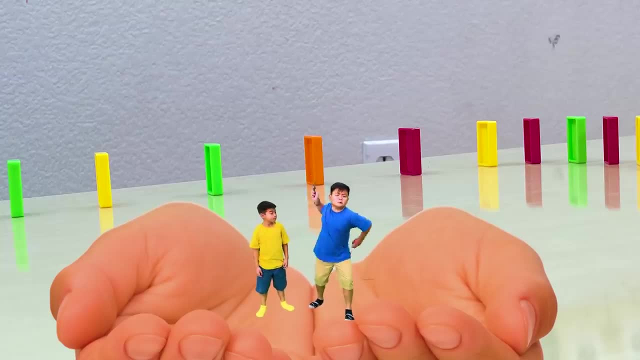 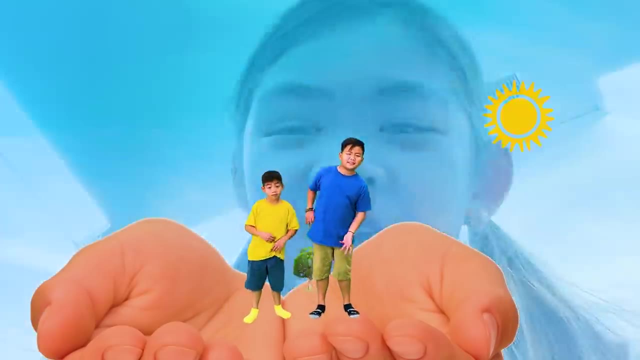 Oh, cute Bugs. We're not bugs. Huh, You're kids. We don't mean any harm, We just need the sun. People, plants and animals on the earth need the sun to thrive. Thank you for teaching me about science, Alex. Why don't you? 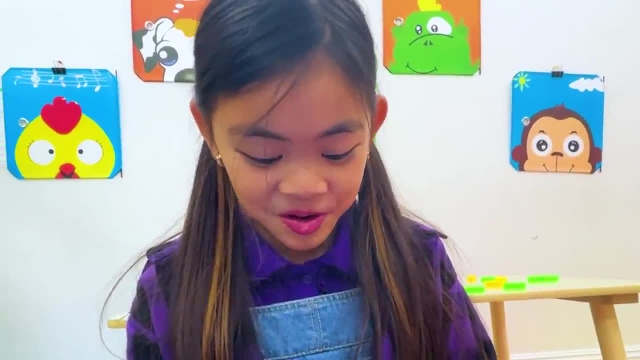 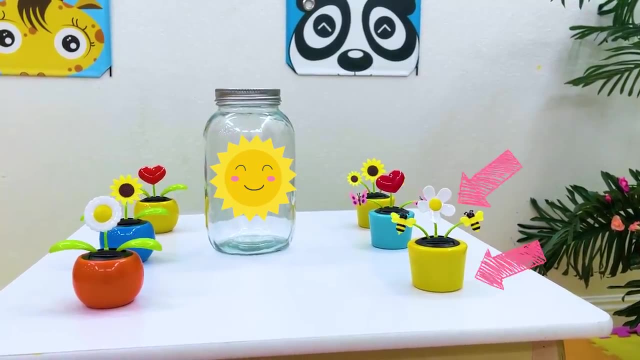 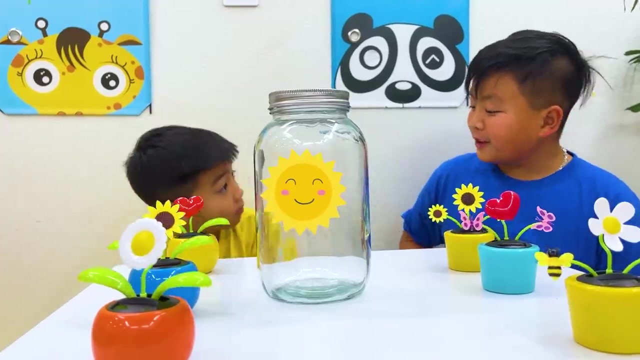 take the sun anyway. Only the coolest toys ever. Let me show you How does this toy work. The pedals swing with the magnet in the base. When the sun hits the toy, electricity is sent through a coil that interacts with the magnet. Whoa, we learned a lot. 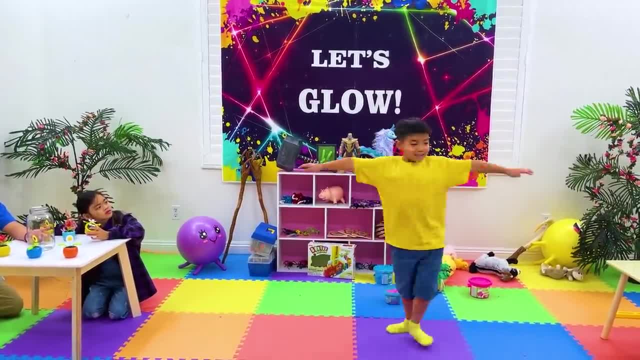 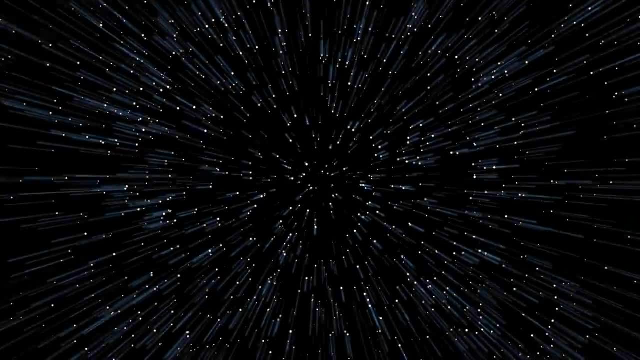 It's my turn to be the teacher. Wow, Eric, you're a star. So is the sun. The sun is a star in the center of our solar system. There are billions of stars in the galaxy, but ours is special: It is the most important source of energy. 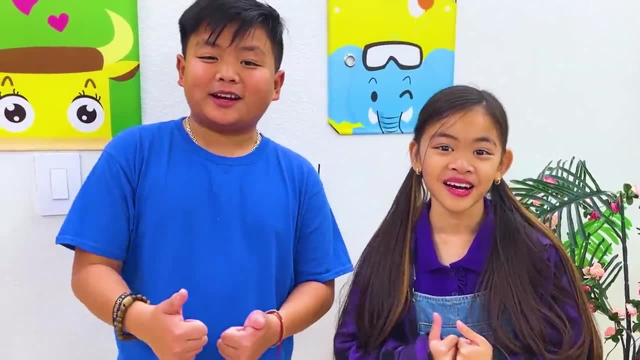 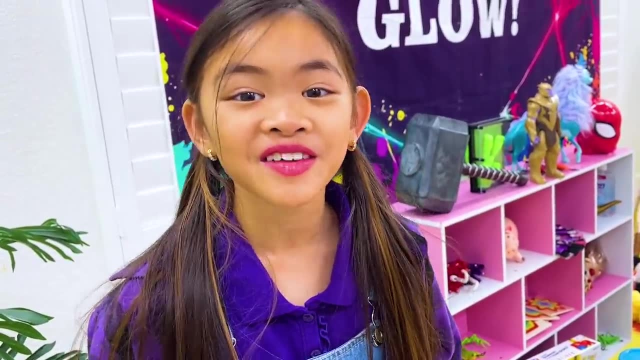 that's in life on earth. Wow, that's really interesting, Eric. Okay, we're on our way. We had a lot of fun. It's time to go now. Thanks for visiting me. I'll come visit you next time. 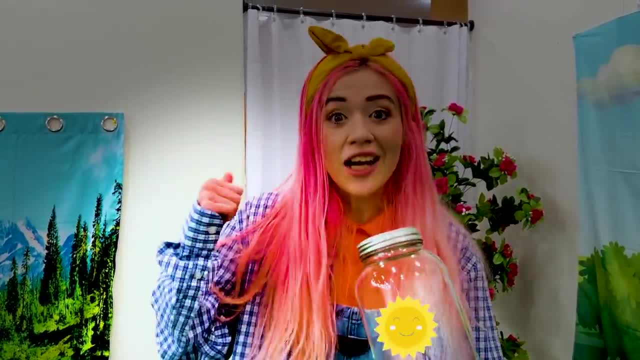 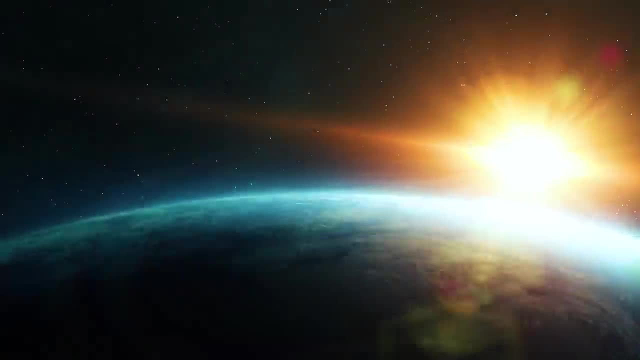 We got the sun back. Great job. kids, Take it outside and let it out safely. Are you ready? Yeah, Whoa, Wow, Yay. Video off camera. Bye.